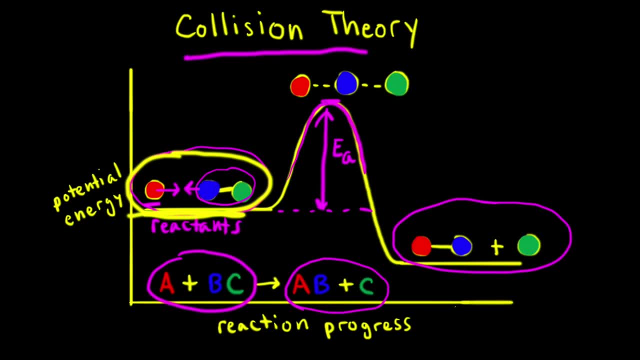 each other and our reaction never occurs. So let's look at the reaction on the left side of the hill to overcome this activation energy barrier. As an analogy, let's think about hitting a golf ball. So let's imagine we have a hill, and on the right, 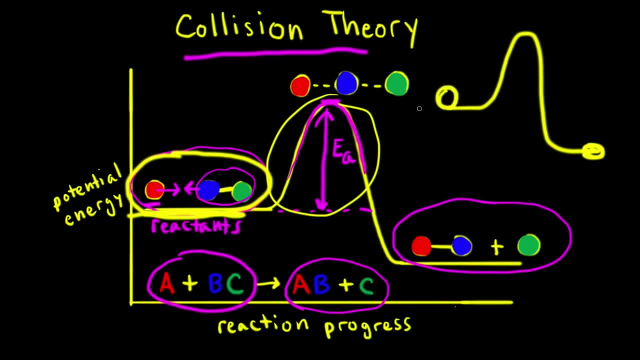 side of the hill. somewhere is the hole down here, and on the left side of the hill is our golf ball. So we know we have to hit this golf ball with enough force to give it enough kinetic energy for it to reach the top of the hill and to roll over the hill and go into the hole. So we can imagine. we can imagine this hill as being a hill of potential energy. 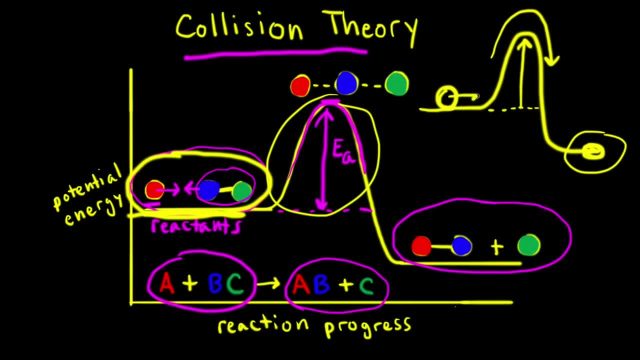 And this golf ball needs to have enough kinetic energy to turn into enough potential energy to go over the hill. If we don't hit our golf ball hard enough, it might not have enough energy to go over the hill. So if we hit it softly it might just roll halfway up the hill and roll back down again. 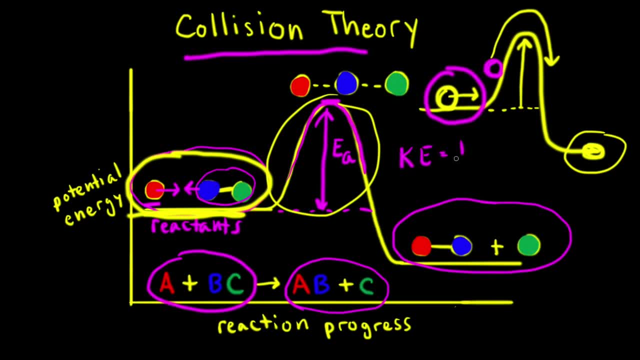 Kinetic energy is equal to one half mv squared. So m would be the mass of the golf ball and v would be the velocity of the ball. So we have to hit it with enough force so it has a high enough velocity to have a high enough kinetic energy to get over the hill. 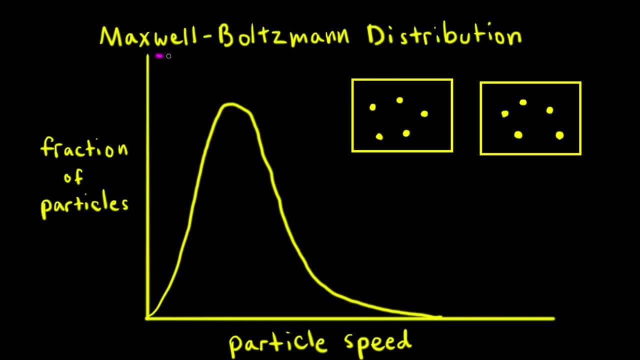 Let's apply collision theory to a Maxwell-Boltzmann distribution. Usually, a Maxwell-Boltzmann distribution has fraction of particles or relative numbers of particles on the y-axis and particle speed on the x-axis, And a Maxwell-Boltzmann distribution shows us the range of speed. 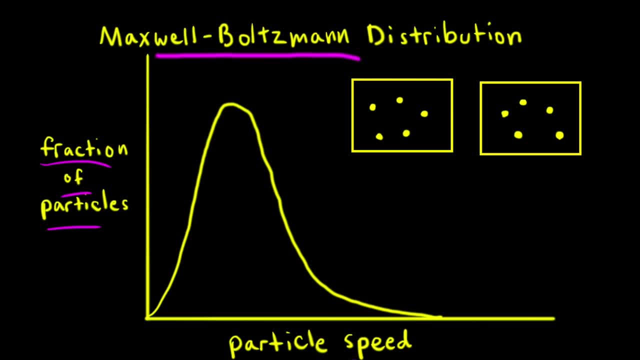 So let's say we have a sample of gas at a particular temperature, T. These particles aren't traveling at the same speed. There's a range of speeds available to them, So one particle might be traveling really slowly. so we'll draw a very short arrow here. 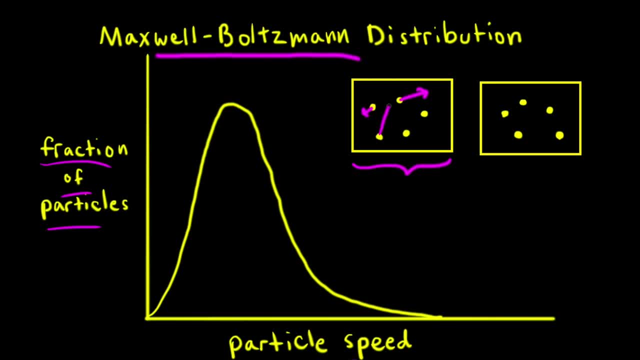 A few more might be traveling a little faster, so we'll draw the arrow longer to indicate a faster speed. And maybe one particle is traveling the fastest, so we'll give this particle the longest arrow. We can think about the area under the curve for a Maxwell-Boltzmann distribution as representing all of the particles in our sample. 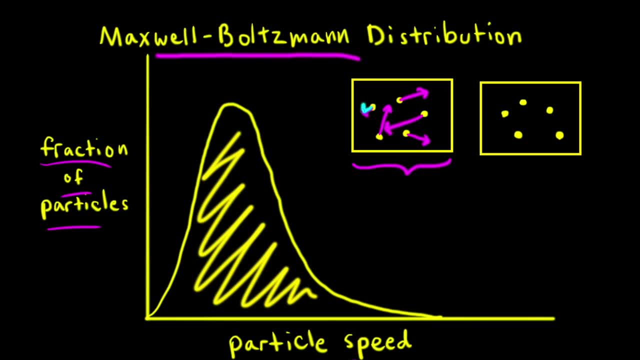 So we had this one particle here moving very slowly, And so if we look at our curve and we think about the area under the curve that's at a low particle speed, this area is smaller than other parts of the curve, So that's represented here by only this one particle moving very slowly. 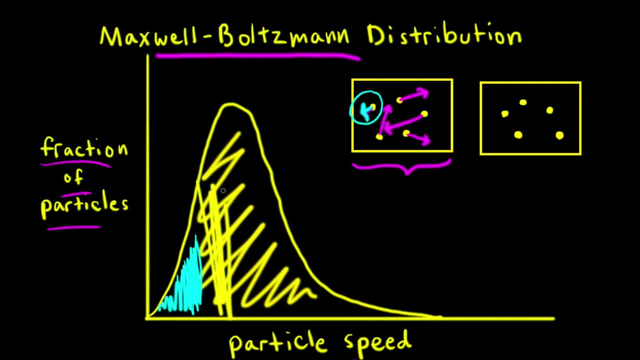 If we think about this next part of the curve, this is a large amount of area in here And these particles are traveling at a higher speed. So maybe these three particles here would represent the particles moving at a higher speed. And then finally, we had this one particle here. We drew this arrow longer than the others. 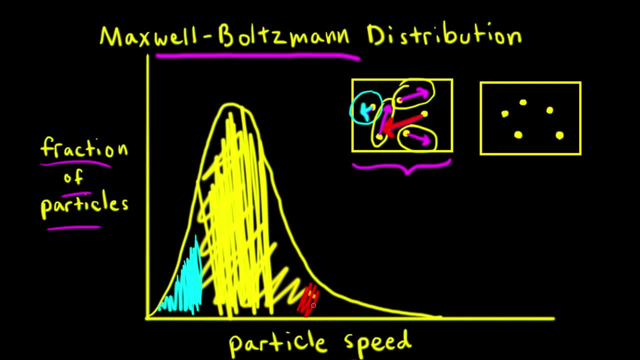 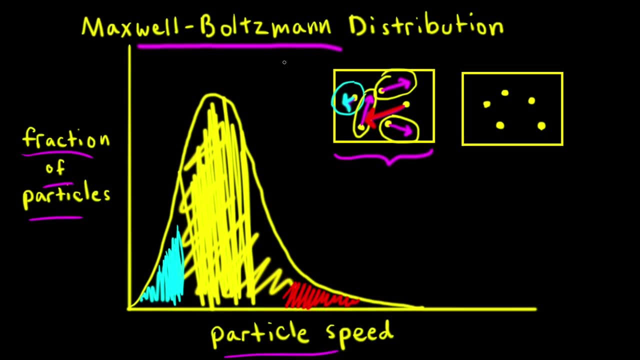 So this particle is traveling faster than the other one, So maybe this area under the curve up here is represented by that one particle. We know from collision theory that particles have to have enough kinetic energy to overcome the activation energy for a reaction to occur. 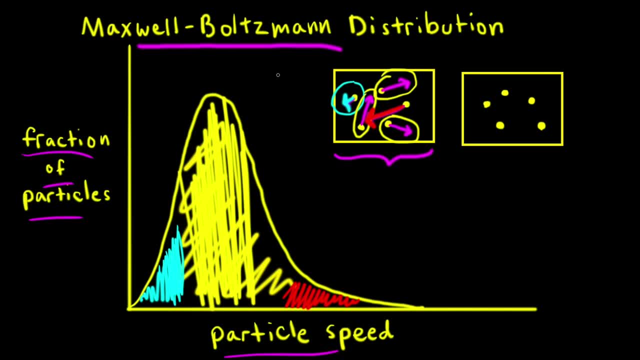 So we can draw a line representing the activation energy on a Maxwell-Boltzmann distribution. So if I draw this line, this dotted line right here, this represents my activation energy And instead of particle speed, you could think about the x-axis as being kinetic energy, if you want. 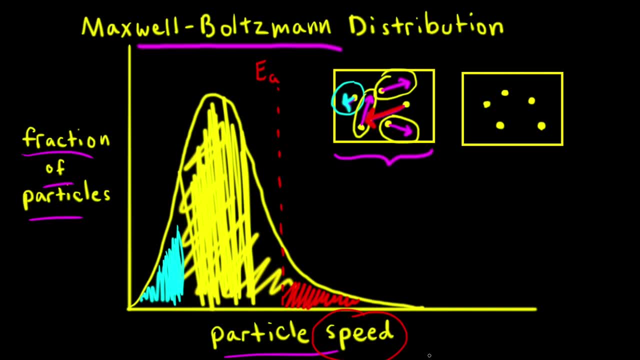 So the higher, the faster a particle is traveling, the higher its kinetic energy. And so the area of the curve, the area under the curve, to the right of this dashed line, this represents all of the particles that have enough, that have enough kinetic energy for this reaction to occur. 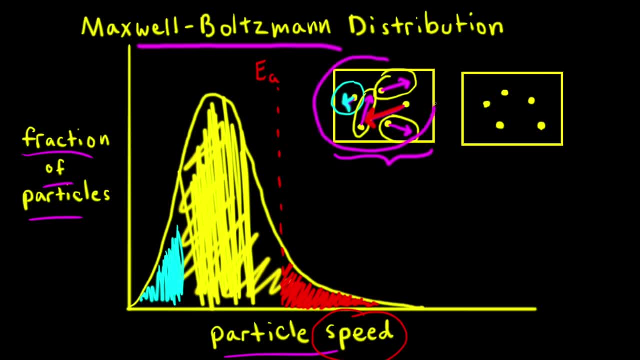 Next, let's think about what happens to the particles in our sample when we increase the temperature. So when we increase the temperature, the Maxwell-Boltzmann distribution changes. So what happens is the peak height drops and our Maxwell-Boltzmann distribution curve gets broader. 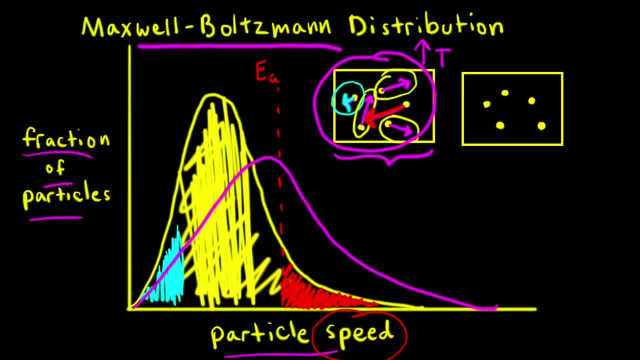 So it looks something like this at a higher temperature. So we still have some particles traveling at relatively low speeds. right, Remember, it's the area under the curve, So maybe that's represented by this one particle here. And next let's think about the area to the left of this dashed line for Ea.